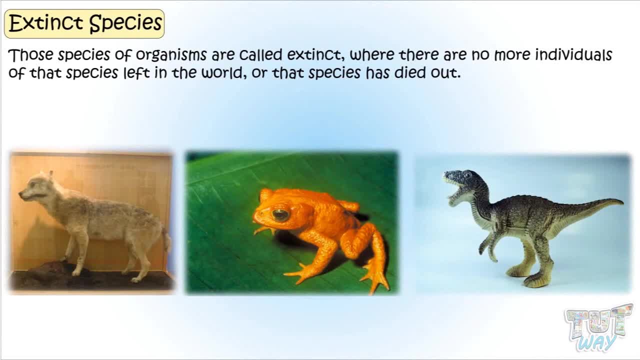 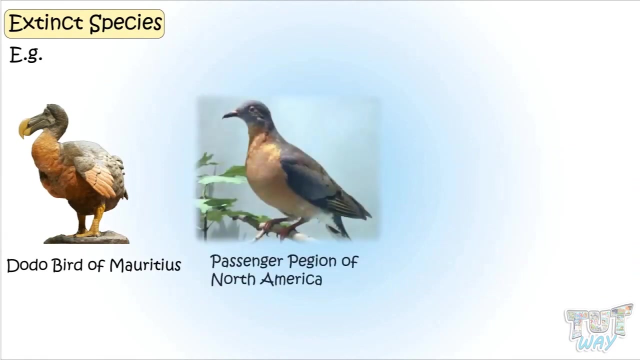 that species left in the world or that species is died out. Millions of species that ever lived on earth have gone extinct by now. That is, our earth is deprived of so many beautiful species. Now let's look at a few examples: Dodo bird of Mauritius. passenger pigeon of North America. 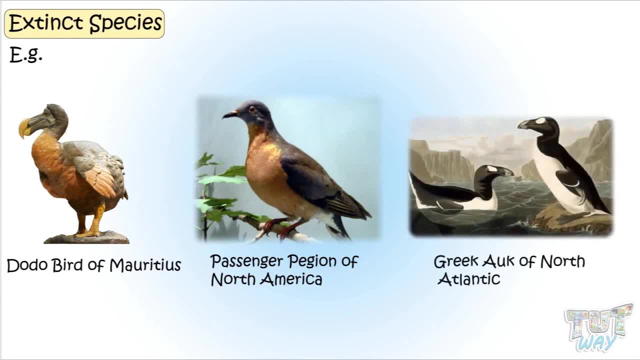 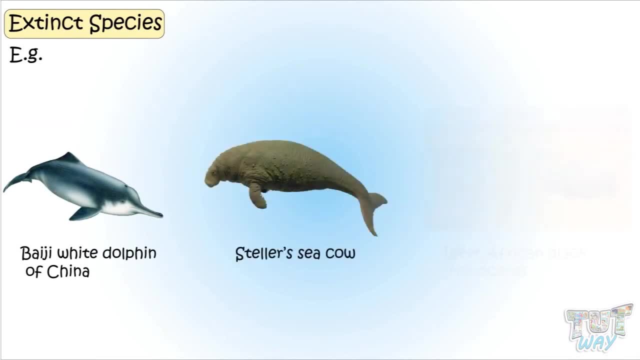 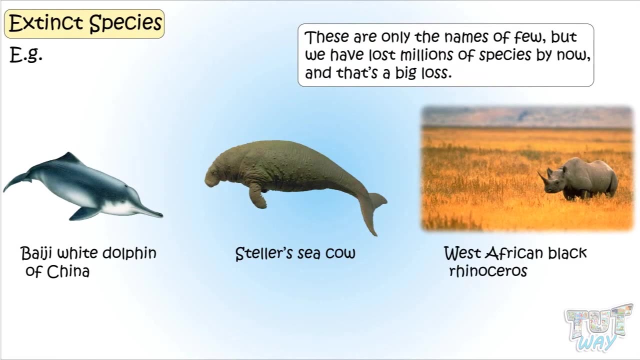 Greek auk of North Africa, Atlantic Baiji, white dolphin of China, Cellar sea cow, West African black rhinoceros- These are only to name a few, but we have lost a million of species by now and that's a big loss. 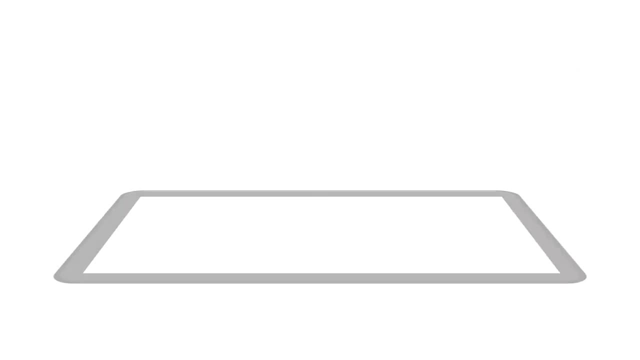 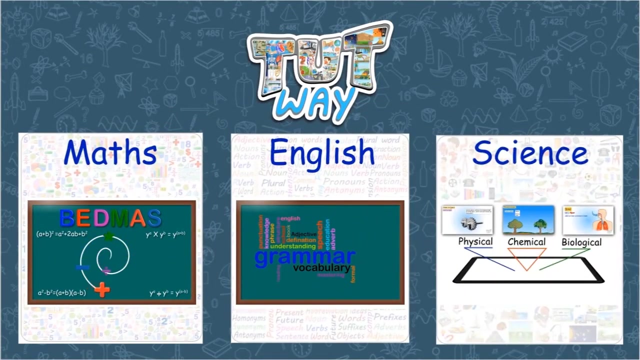 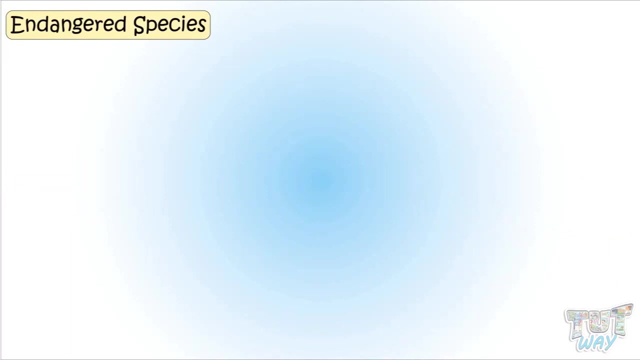 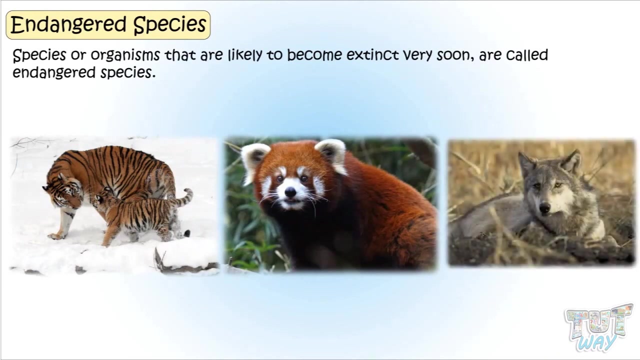 TootWay has thousands of animated videos on math, English and science to clear the core basics of these subjects. Now let's see what are endangered species. Species of organisms that are likely to become extinct very soon are called endangered species. These are the species. 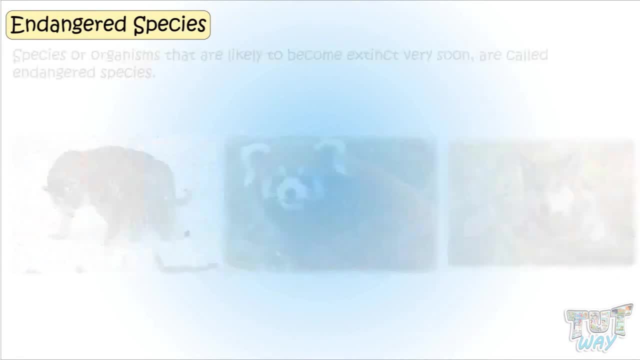 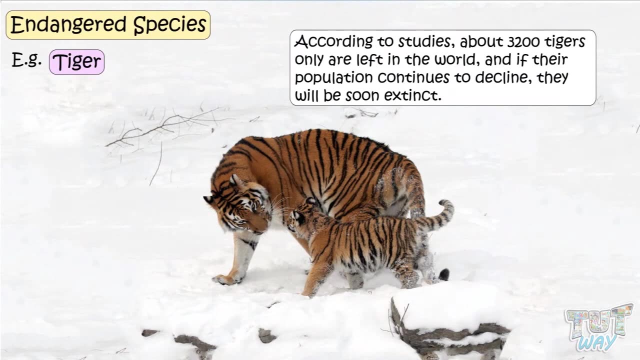 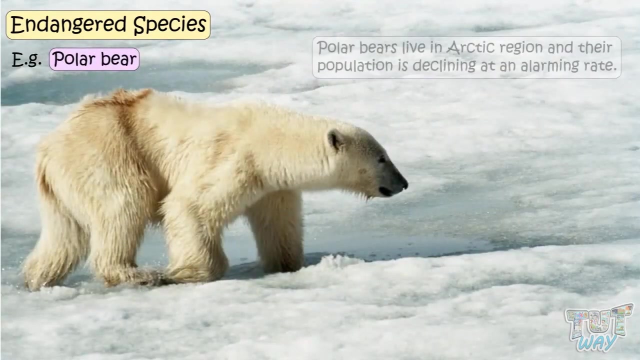 we can save from extinction. Example: tiger. According to studies, about 3,200 tigers only are left in the world and if their population continued to decline, they will be soon extinct. Polar bears. Polar bears live in Arctic regions and their population is declining at an alarming. 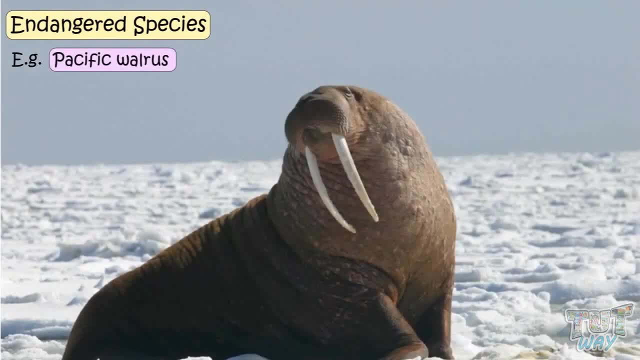 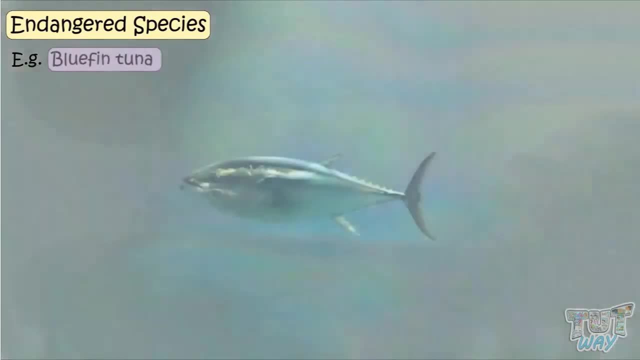 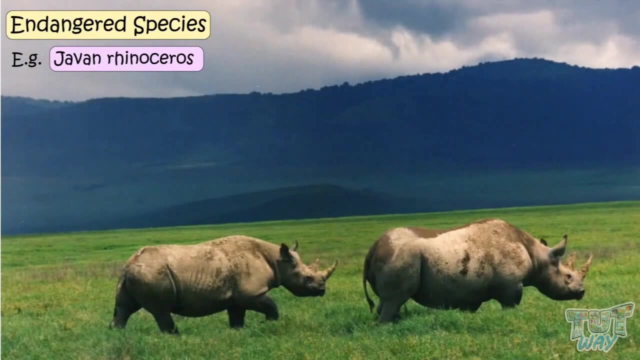 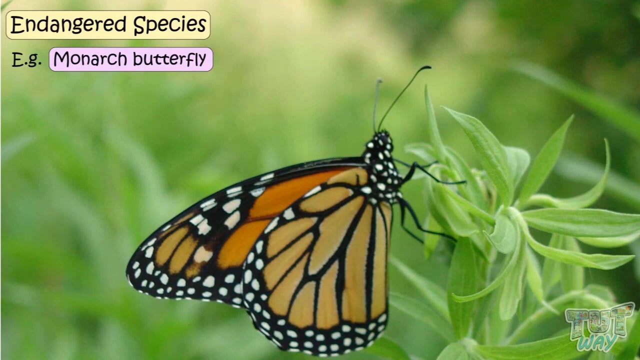 rate, Pacific Pacific walrus, Magellanic penguin, leatherback turtle, bluefin tuna, mountain gorilla, Javan, rhinoceros, giant panda, monarch butterfly and many more. These are just a few to be named. We need. 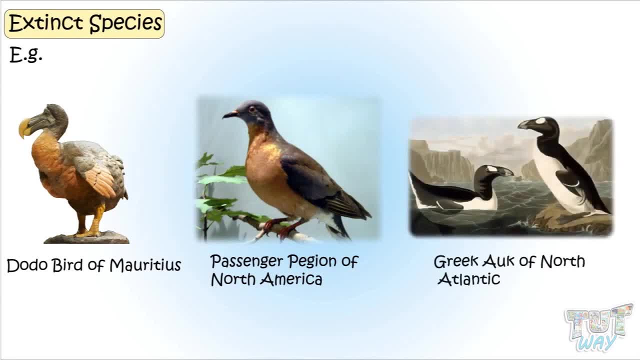 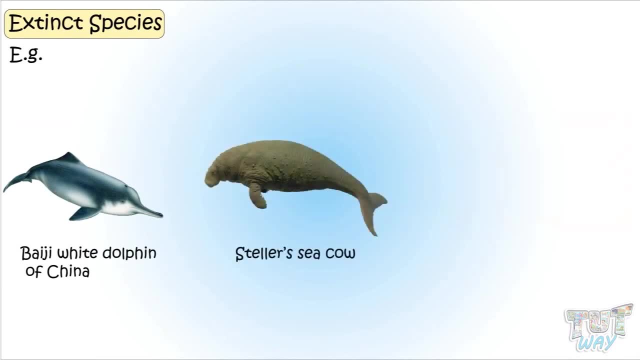 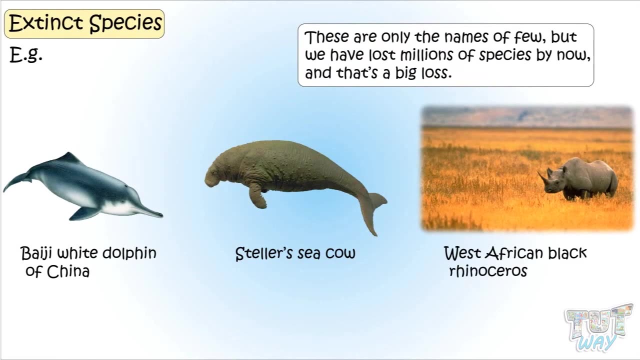 Greek auk of North Africa, Atlantic Baiji, white dolphin of China, Cellar sea cow, West African black rhinoceros- These are only to name a few, but we have lost a million of species by now and that's a big loss. 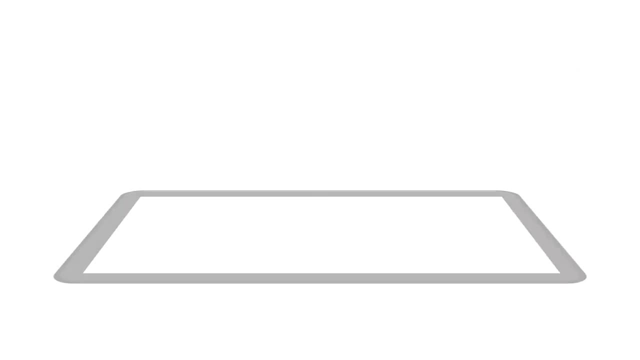 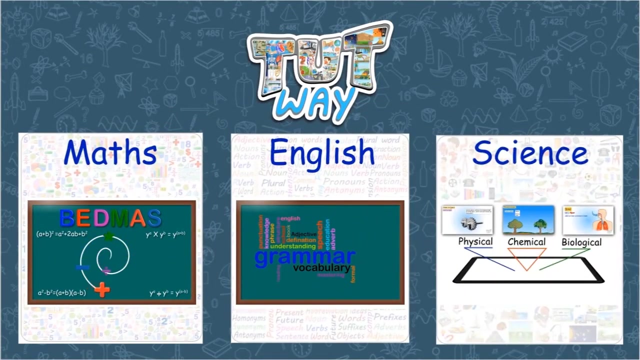 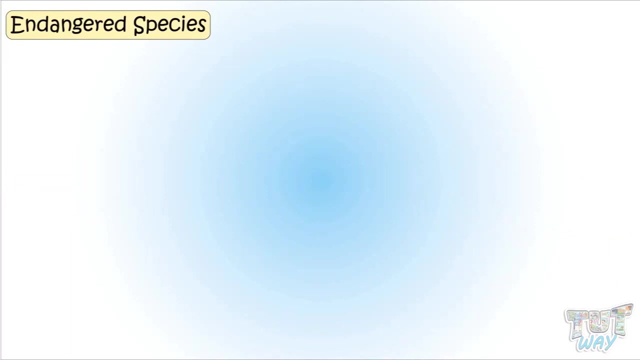 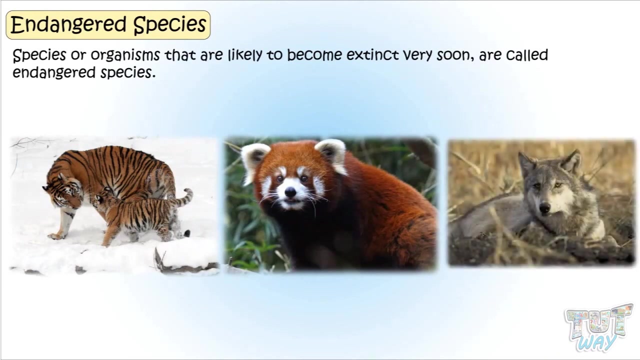 TootWay has thousands of animated videos on math, English and science to clear the core basics of these subjects. Now let's see what are endangered species. Species of organisms that are likely to become extinct very soon are called endangered species. These are the species. 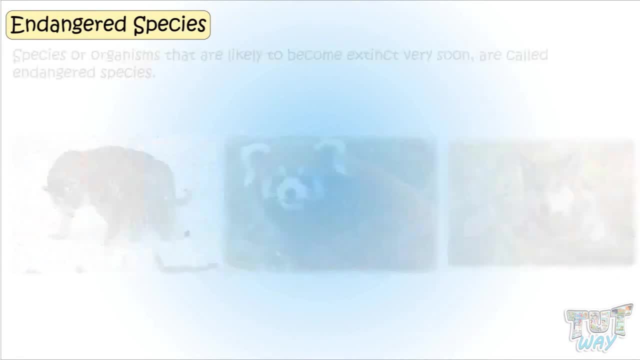 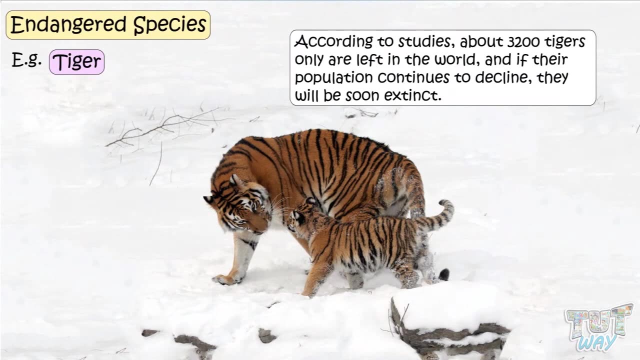 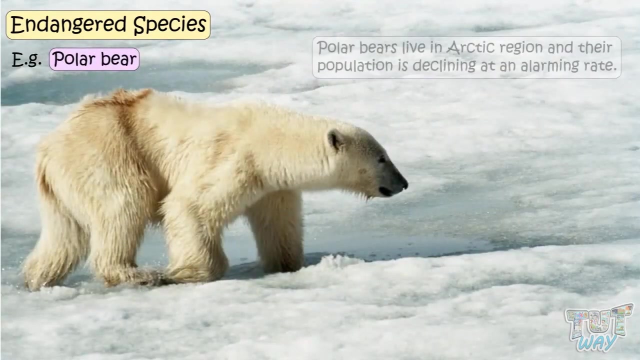 we can save from extinction. Example: tiger. According to studies, about 3,200 tigers only are left in the world and if their population continued to decline, they will be soon extinct. Polar bears. Polar bears live in Arctic regions and their population is declining at an alarming. 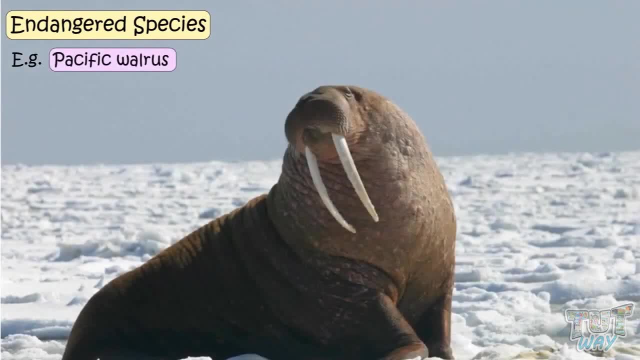 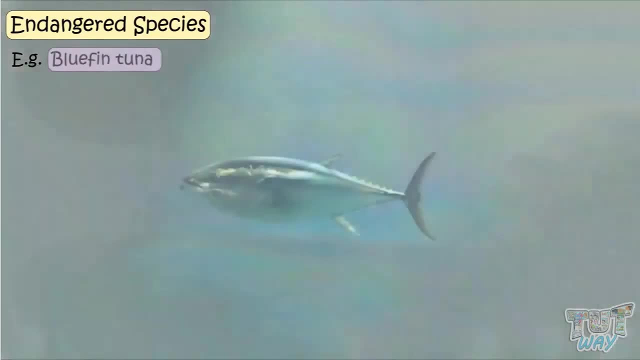 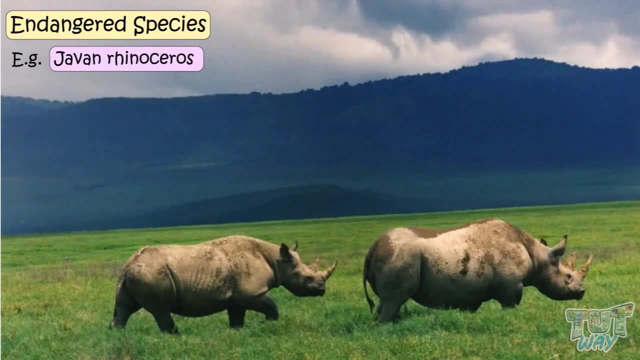 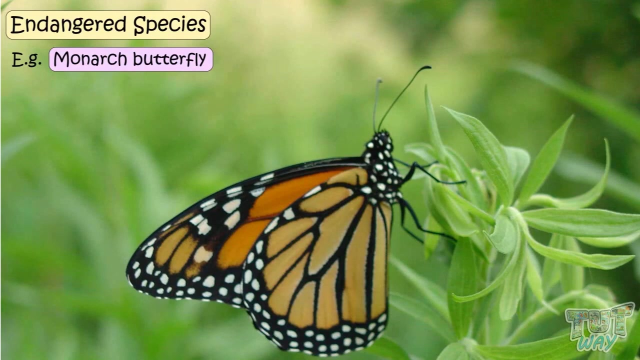 rate, Pacific walrus, Magellanic penguin, Leatherback, turtle, Bluefin, tuna, Mountain gorilla, Javan rhinoceros, Giant panda, Monarch, butterfly and many more. These are just a few to be named. We. 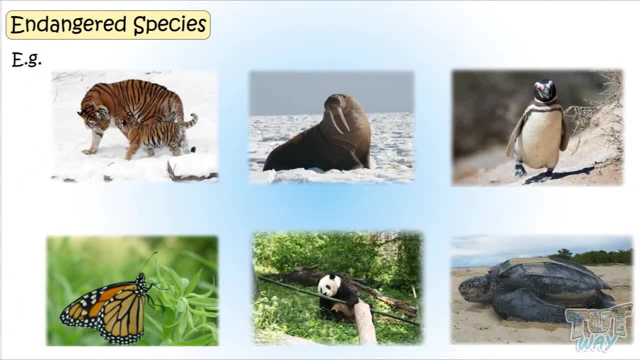 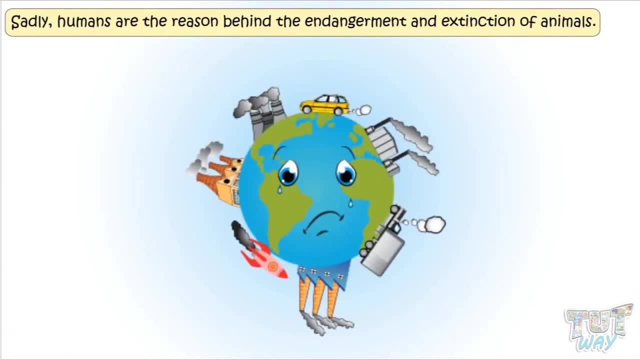 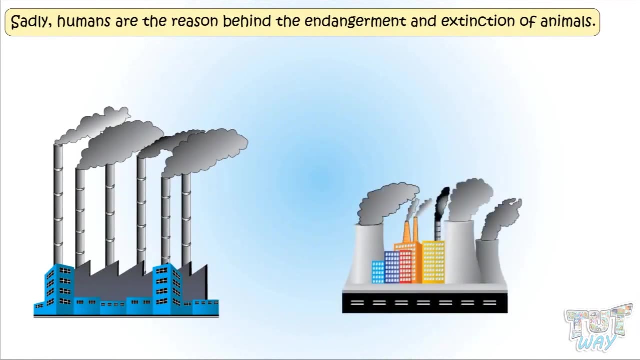 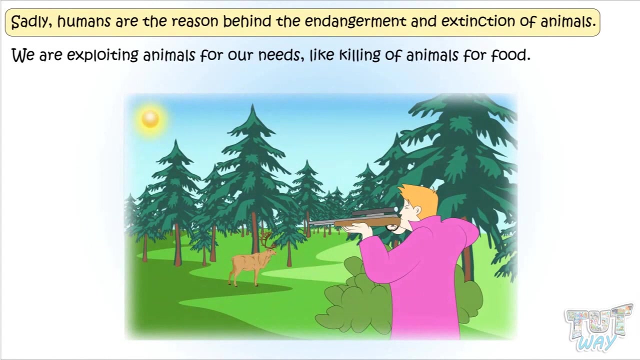 need to save them or they will soon disappear, Be extinct Kids. The most sad part is that the main reason behind endangerment and extinction of species is humans, that is, we and our development activities. We are exploiting animals for our needs, like killing animals for food. We are destroying their natural 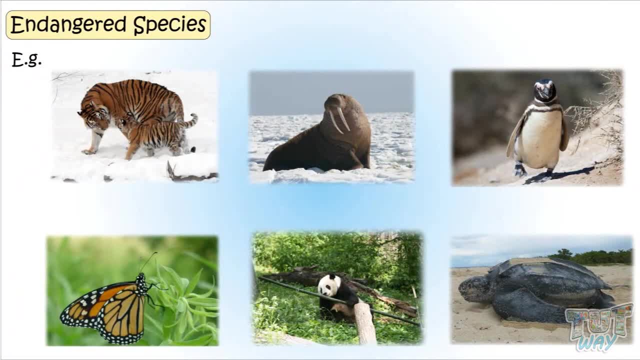 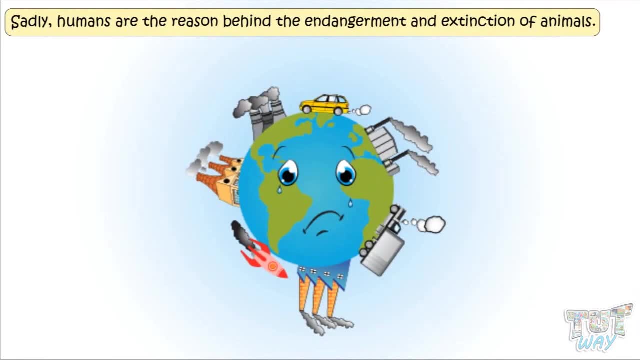 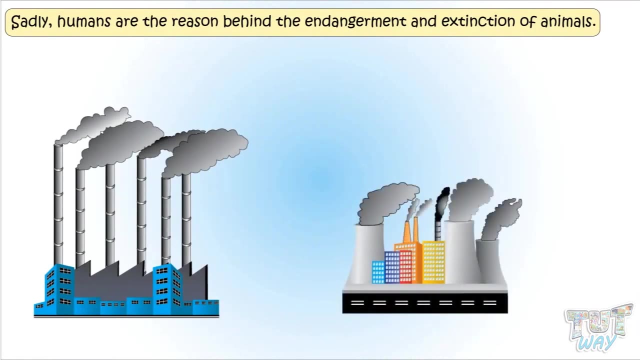 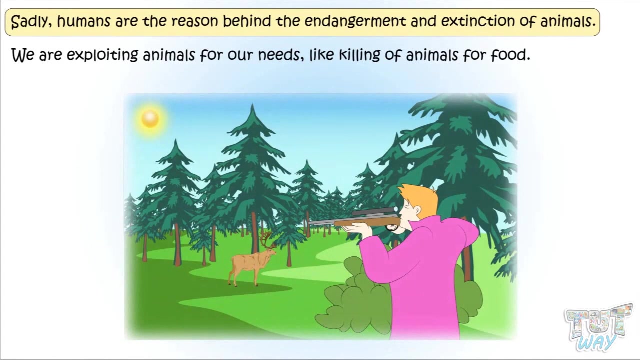 to save them, or they will soon be extinct. Kids. The most sad part is that the main reason behind endangerment and extinction of species is humans, that is, we and our development activities. We are exploiting animals for our needs, like killing animals for food. We are destroying their natural habitat for our development activities. 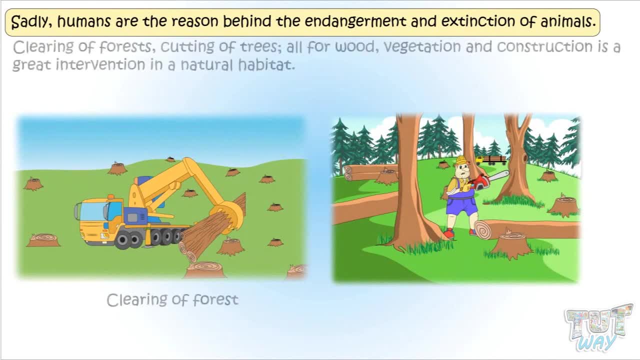 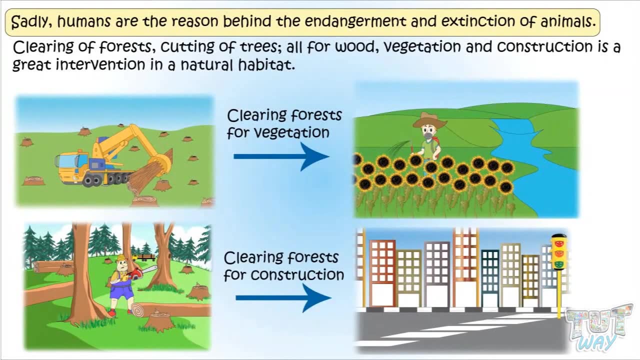 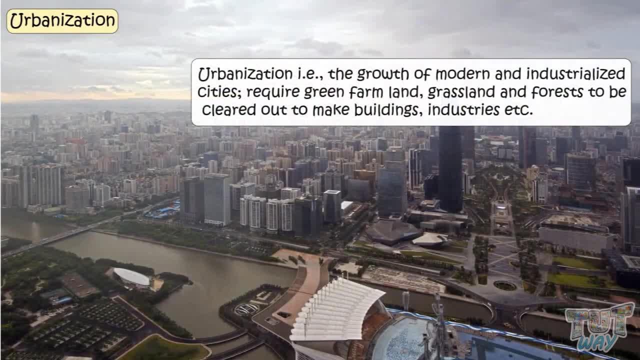 Urbanization. Urbanization, That is the growth of modern industrialized cities. All require green farmland, grasslands, forests to be cleared out to make buildings. All require green farmland, grasslands, forests to be cleared out to make buildings. 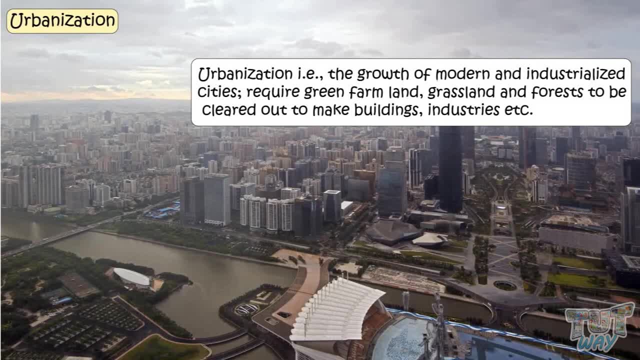 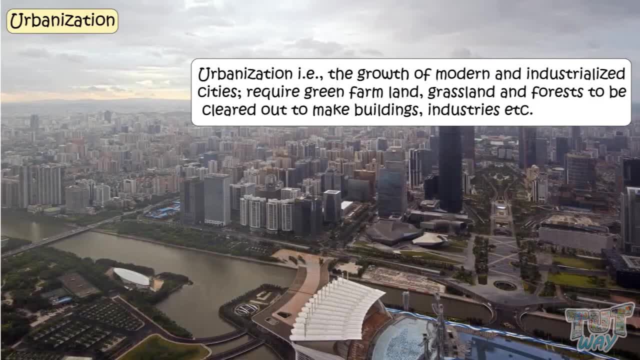 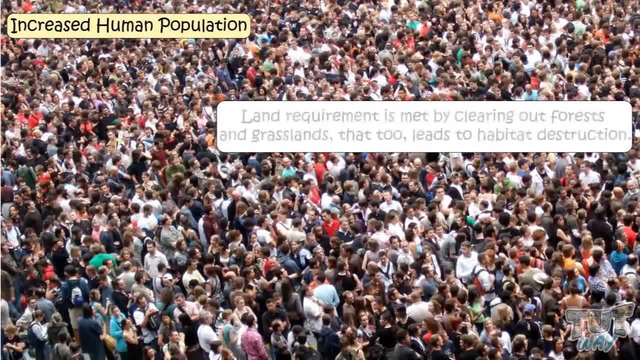 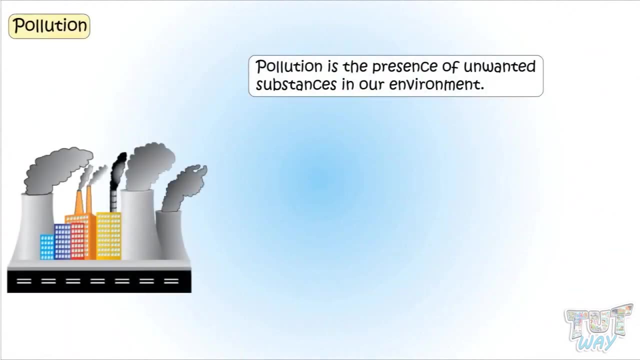 land and land requirement is met by clearing out forests and grasslands, and that too leads to habitat destruction. We learnt urbanization and increasing population are leading to the loss of habitats. Another reason is pollution. Pollution is a presence of unwanted substances in our environment, Human and 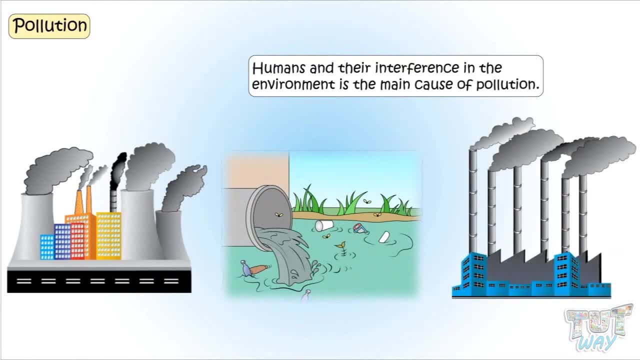 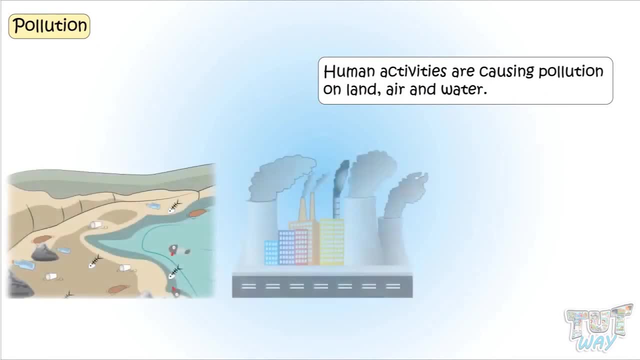 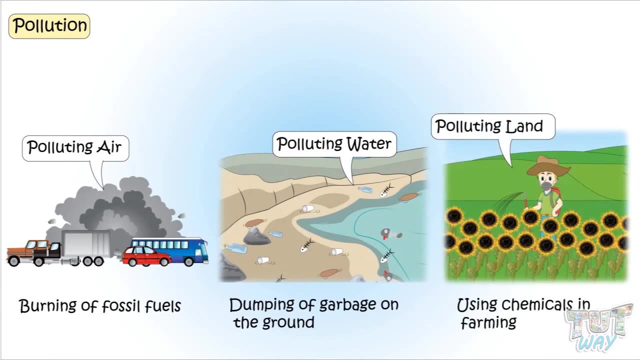 its interference in the environment is the main cause of pollution. Human activities are causing pollution on the land, air and water. Burning of fossil fuels, dumping of garbage on the ground, using chemicals in farming: everything is leading to the pollution of air, water and soil, And this pollution pollutes the 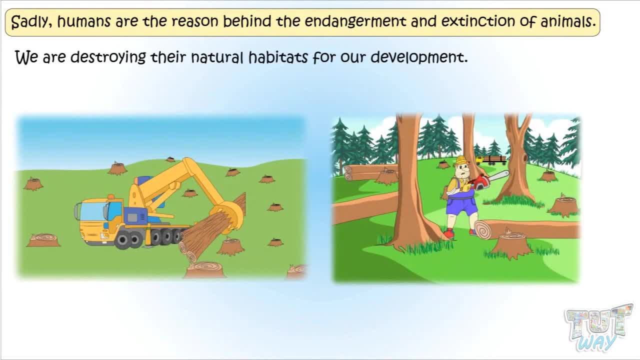 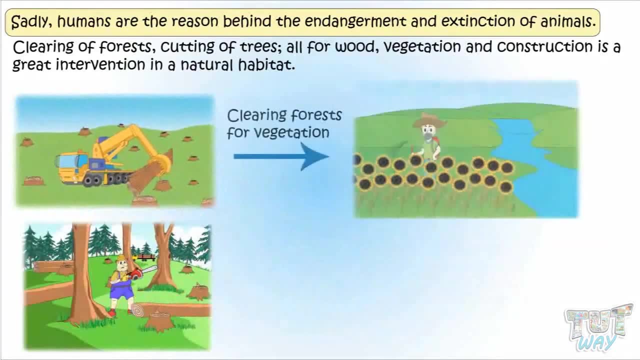 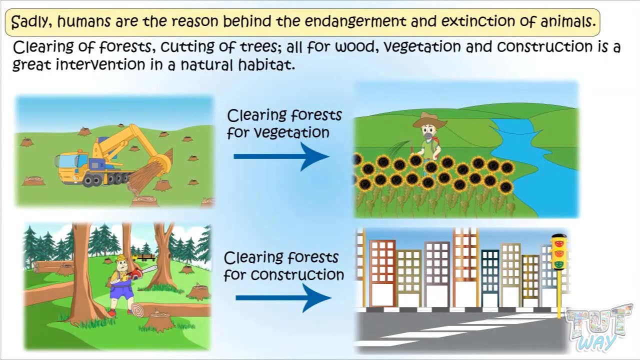 habitat for our development activities. We are destroying their natural habitat for our development activities. We are destroying their natural habitat for our development activities of forests. cutting of trees, all for wood vegetation and construction, is a great intervention in the natural habitats. It is all destroying the natural habitats of animals, because of which. 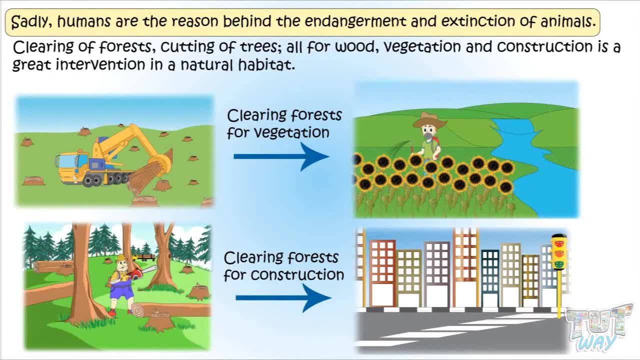 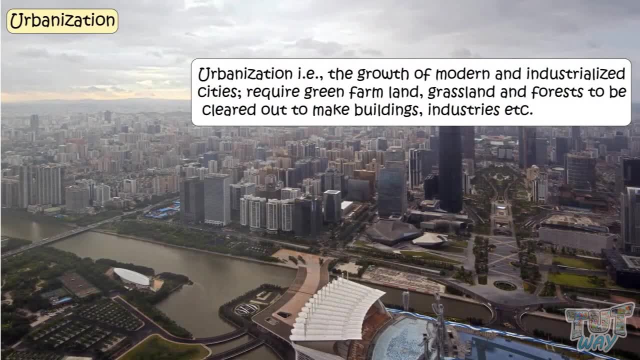 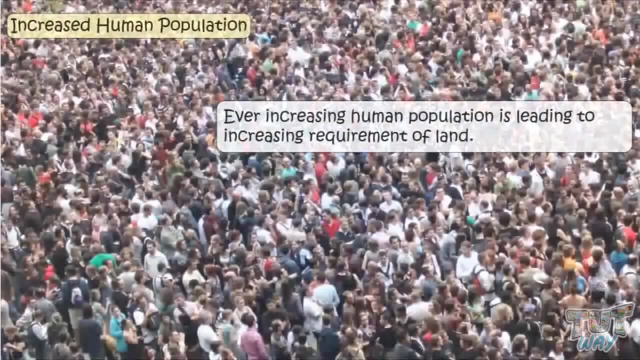 animals are dying out. Urbanization, That is, the growth of modern industrialized cities, All require green farmland, grasslands, forests to be cleared out to make buildings and cities, And all this eventually leads to the loss of natural habitats. Ever-increasing human population is leading to the increasing requirement of land And land. 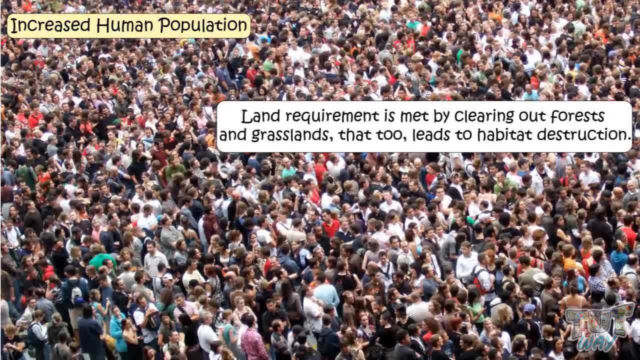 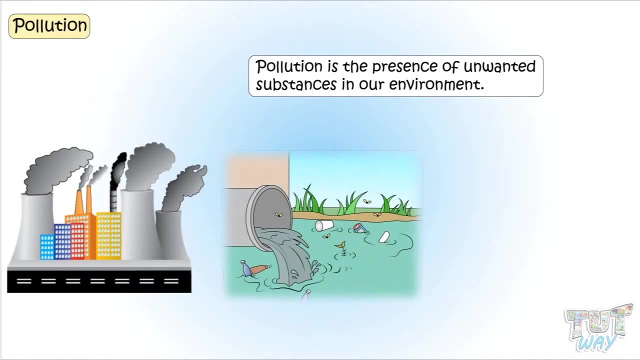 requirement is met by clearing out forests and grasslands, And that too leads to habitat destruction. We learned Earthquake Earthquake. Urbanization and increasing population are leading to the loss of habitats. Another reason is pollution. Pollution is the presence of unwanted substances in our environment. 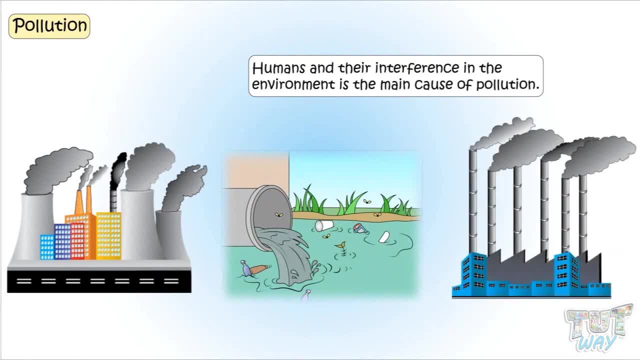 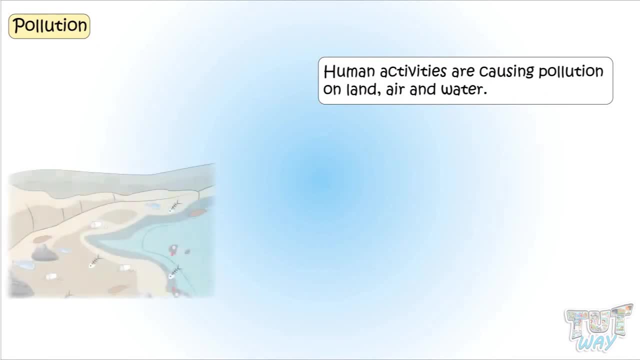 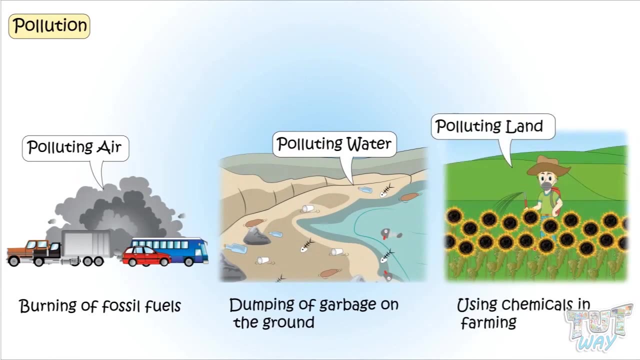 Human and its interference in the environment is the main cause of pollution. Human activities are causing pollution on the land, air and water. Burning of fossil fuels, dumping of garbage on the ground, using chemicals in farming: everything is leading to the pollution of air, water and soil. 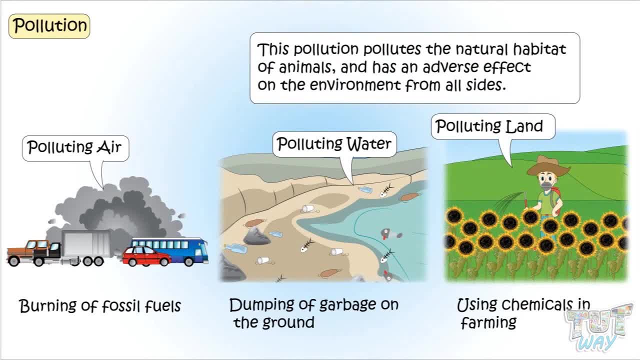 And this pollution pollutes the natural habitats of animals. Pollution has an adverse effect on our environment from all sides. All animals, birds, plants, aquatic life and humans suffer because of this pollution. The biggest example is oil spill. Oil spill- 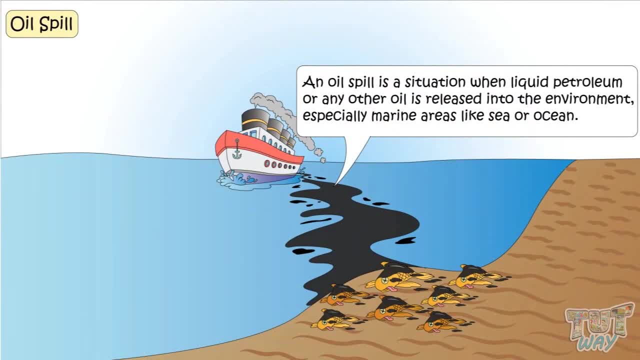 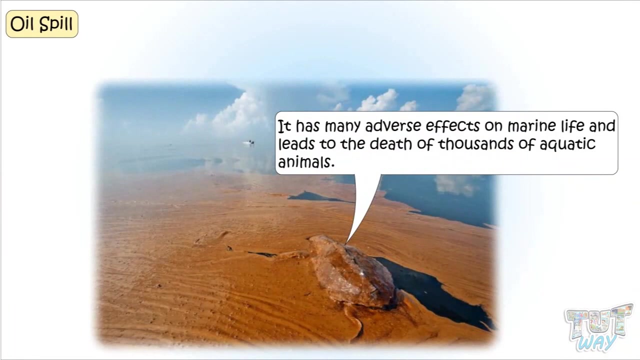 Oil spill is a situation when liquid petroleum or any other oil is released into the environment, especially marine areas, that is, sea or ocean. It can be due to the leakage from some carrier ships or some accident of marine vehicles. It has a very adverse effect on the marine life and this leads to the death of thousands of aquatic animals. 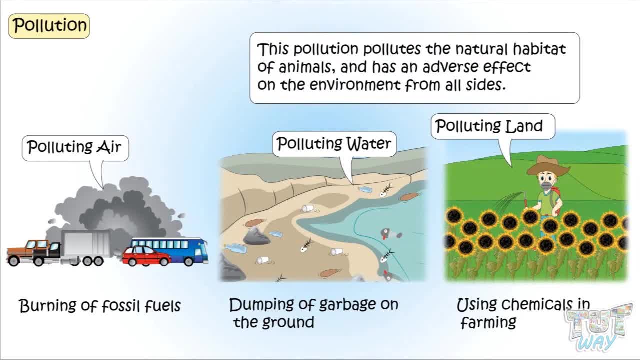 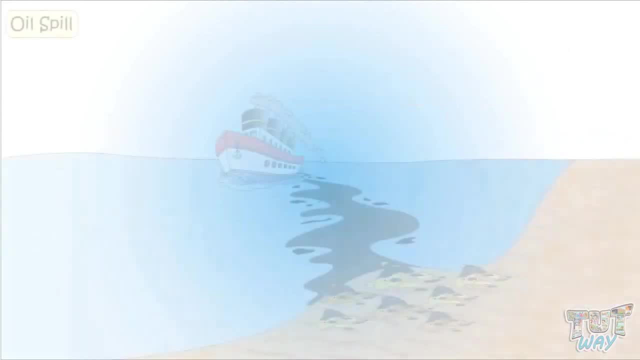 natural habitats of animals. Pollution has an adverse effect on the environment. Pollution has an adverse effect on the environment from all sides. All animals, birds, plants, aquatic life and humans suffer because of this pollution. The biggest example is oil spill. An oil spill. 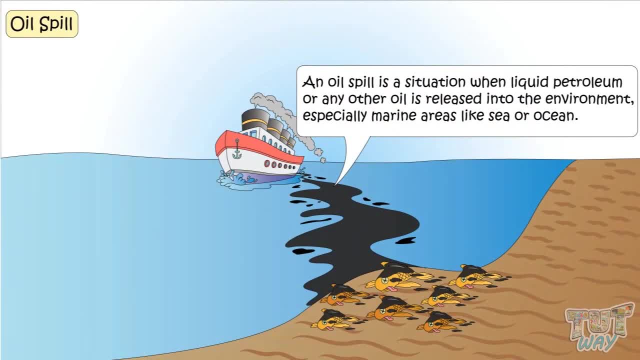 is a situation when liquid petroleum or any other oil is released into the environment, especially marine areas, that is, sea or ocean. It can be due to the leakage of oil, It can be due to leakage from some carrier ships or some accident of marine vehicles. 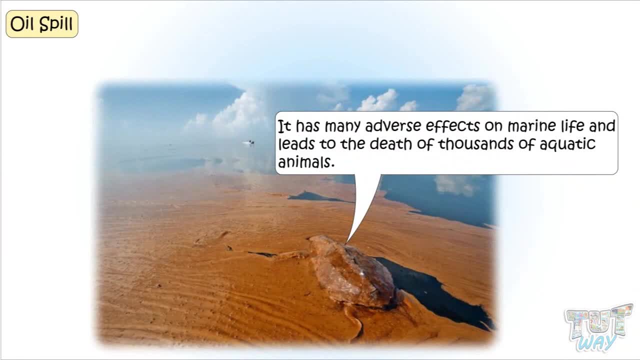 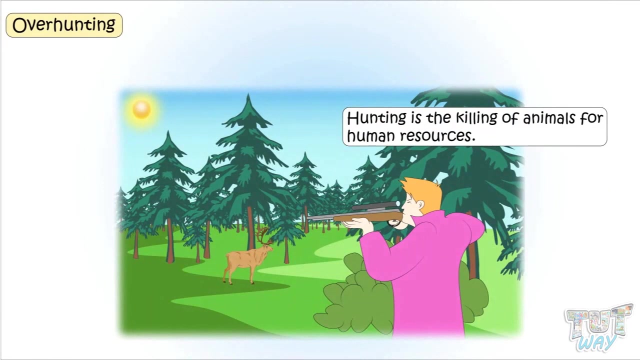 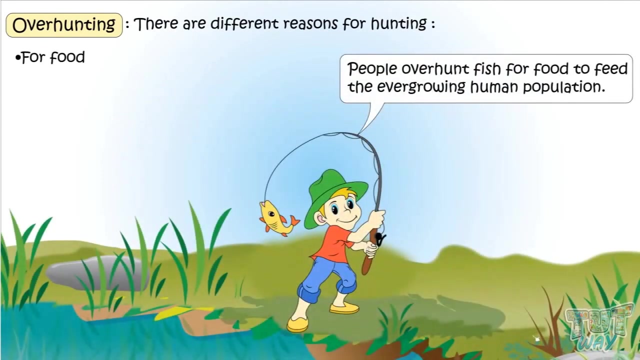 It has a very adverse effect on the marine life and this leads to the death of thousands of aquatic animals. Another important reason for the endangerment and extinction of species is overhunting. Hunting is the killing of animals for human resources. There are different reasons for hunting. It can be food, like people overhunt fish. 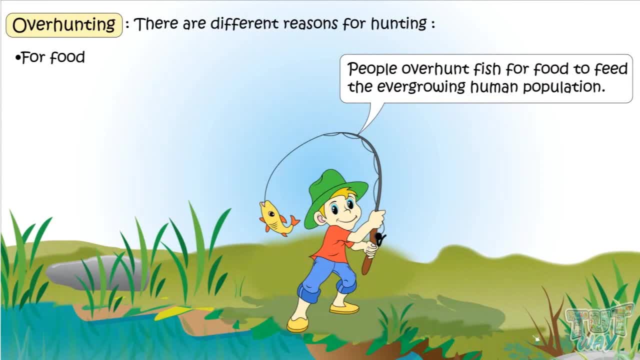 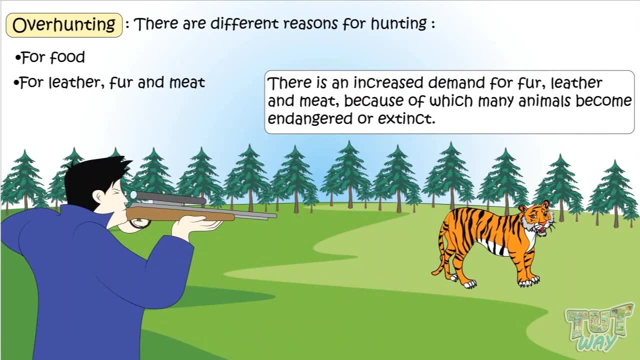 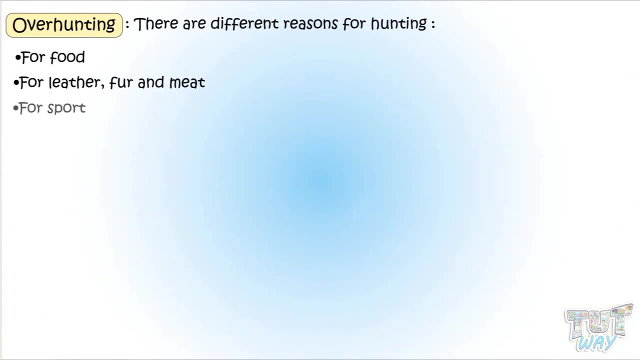 for food to feed the ever-growing human population, Leather or fur. There is an increased demand for fur, leather and meat, because of which many animals become endangered or extinct. even Sports Animal hunting is still considered as a sport in some places, For example, hunting. 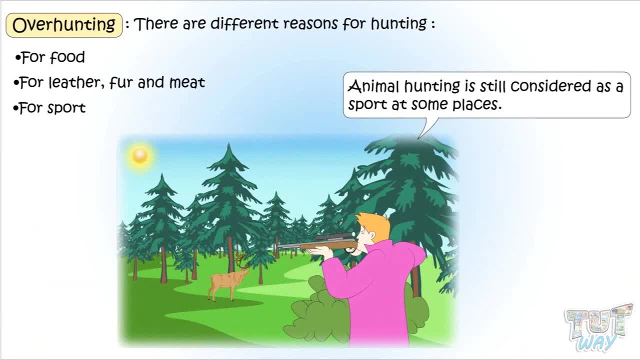 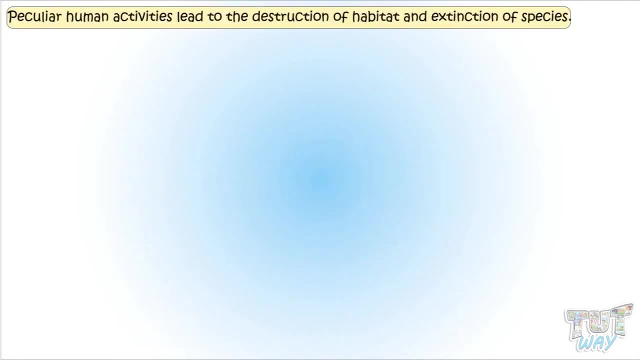 is a major and foremost threat to the declining population of many animal species. Whatever the reason may be, hunting is a major and foremost threat to the declining population of many animal species. Now let's see some peculiar examples of human activities that are leading to habitat destruction. 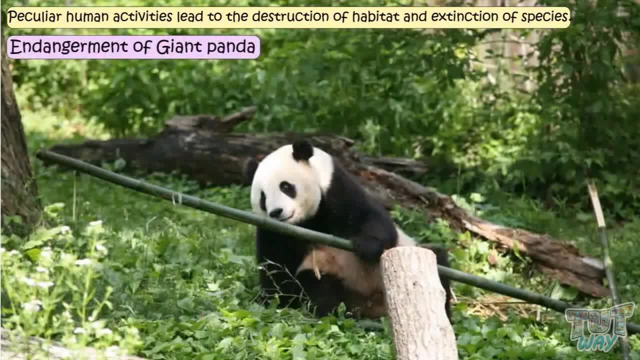 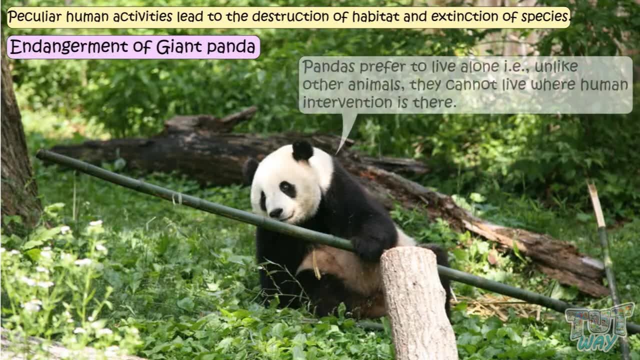 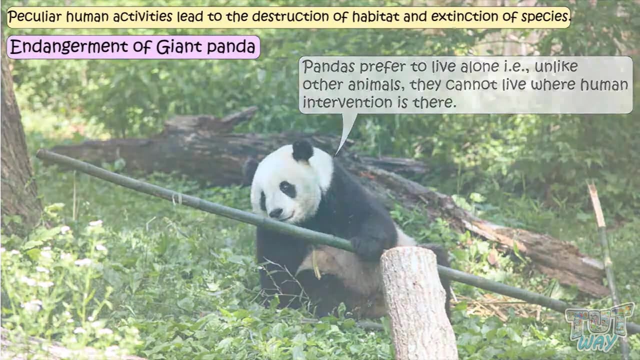 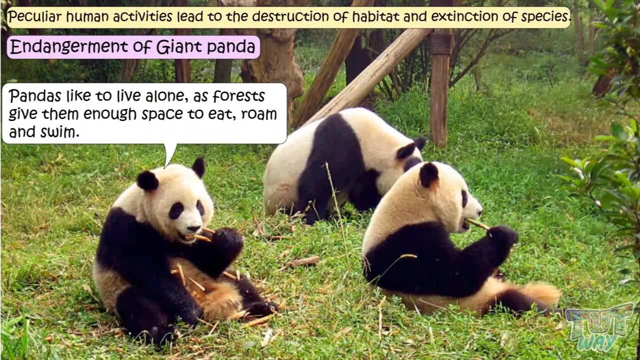 and animal extinction. Giant Panda. Giant pandas only natural habitat is China's mountain forest Pandas prefer to live alone. that is unlike other animals. they cannot live where human intervention is there. Panda like to live alone and forest gives them enough space to eat, roam and swim. 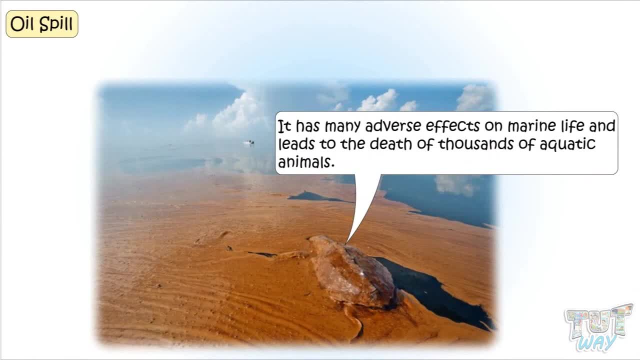 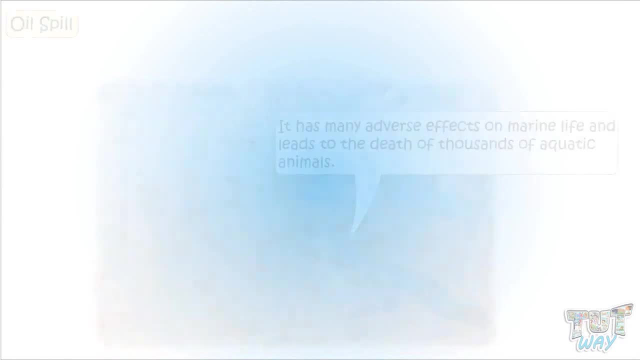 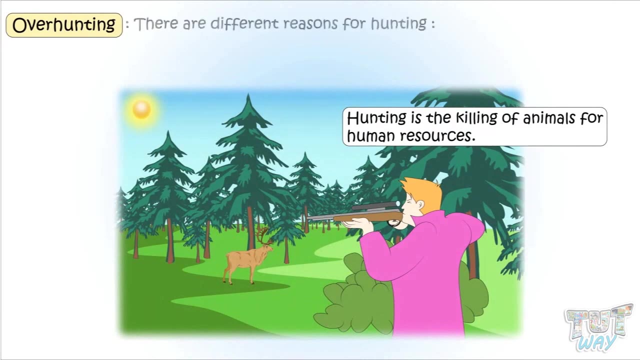 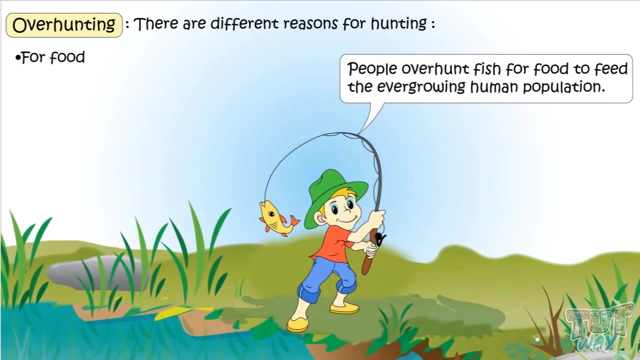 Another important reason for the endangerment and extinction of species is overhunting. Hunting is the killing of animals for human resources. There are different reasons for hunting. It can be food. like people overhunt fish for food to feed the ever-growing human population. 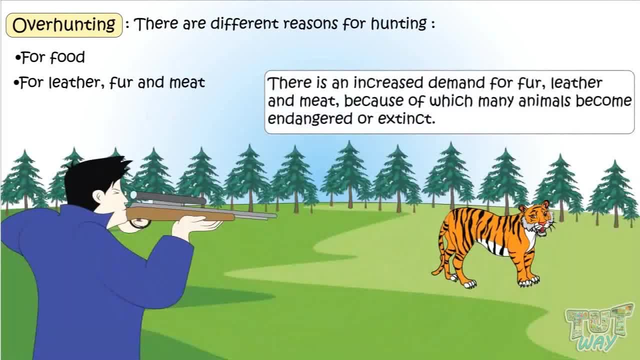 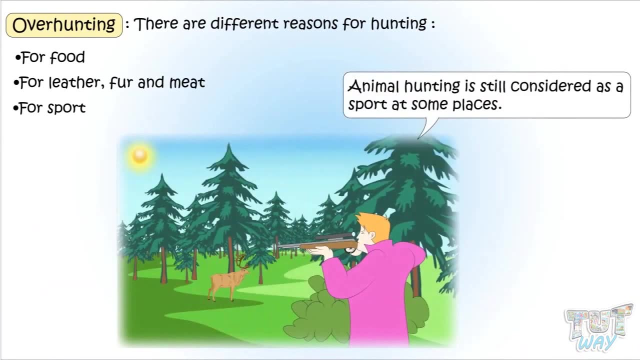 Leather or fur. Leather or fur, There is an increased demand for fur, leather and meat, because of which many animals become endangered or extinct. even Sports: Animal hunting is still considered as a sport in some places, whatever the reason may be, but hunting is a major and foremost threat to the declining population of many animal species. 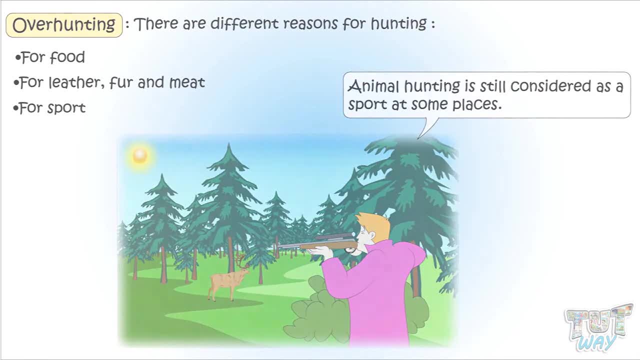 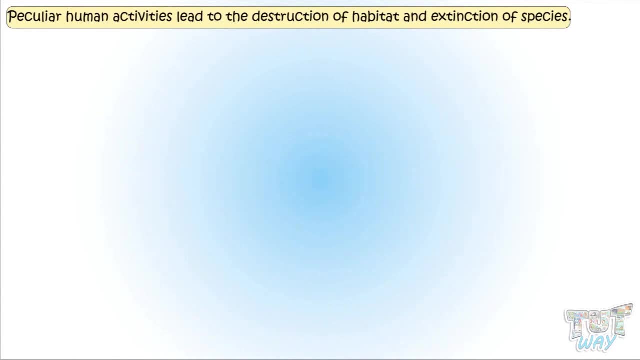 Now let's see some peculiarities of animal hunting. Now let's see some peculiarities of animal hunting. Now let's see some peculiarities of animal hunting. These are some peculiar examples of human activities that are leading to habitat destruction and animal extinction. 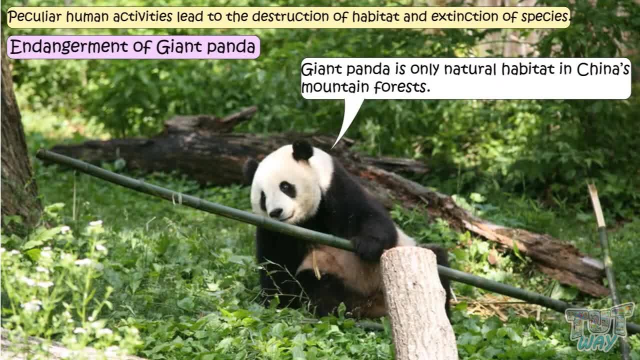 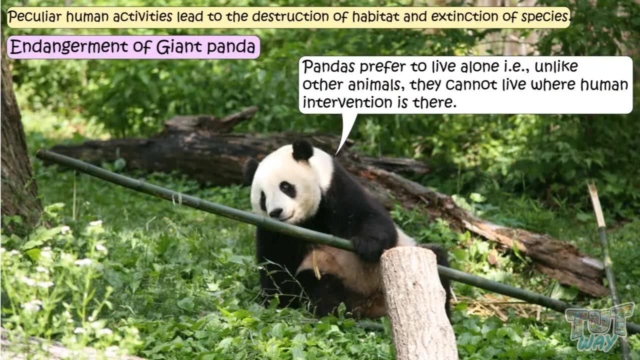 Giant panda. Giant pandas only natural habitat is China's mountain forests. Pandas prefer to live alone. that is unlike other animals. they cannot live where human intervention is there. Pandas like to live alone. Pandas like to live alone, and forest time or time alone is not favourable to them. And forest gives them enough space to eat, eat and suffer. Anarapkae, Anarapkae, Anarapkae, Anarapkae這一 Anarapkae Anarapkae. 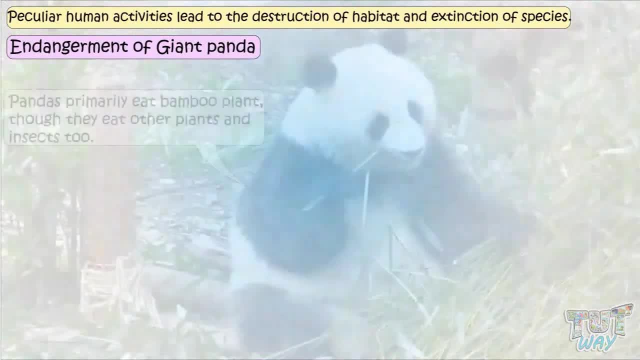 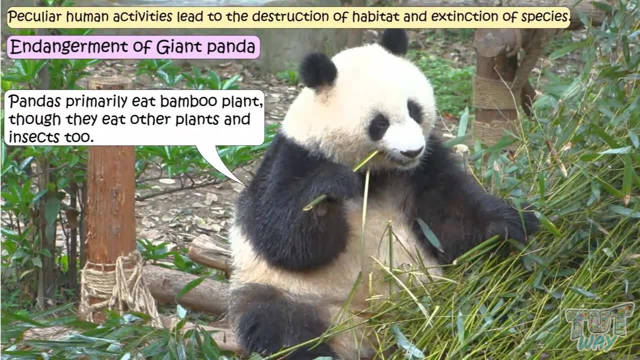 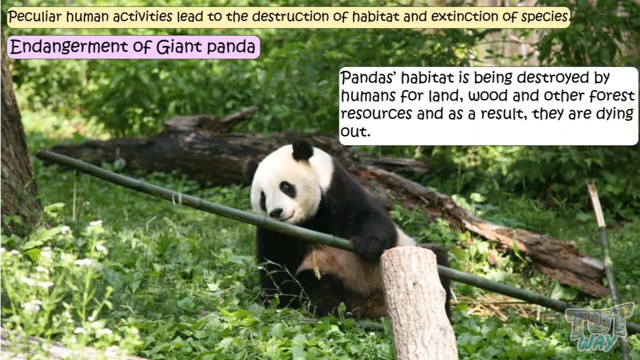 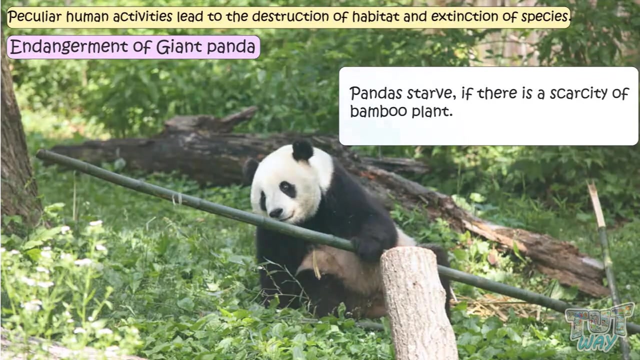 roam and swim and they primarily eat bamboo plant, though they eat other plants and insects too. but pandas habitat is being destroyed by humans for land, wood and other forest resources and, as a result, pandas are dying out. pandas starve if there is a scarcity of bamboo plant. blue whale. the blue whale is a 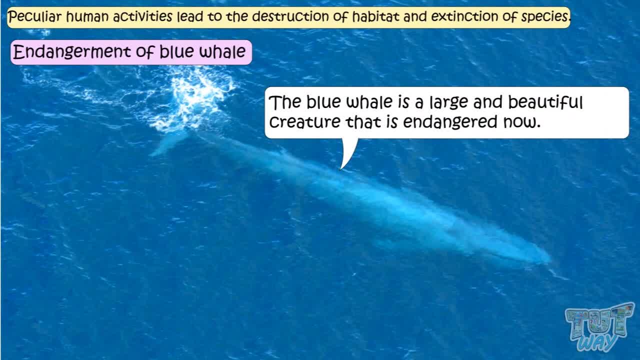 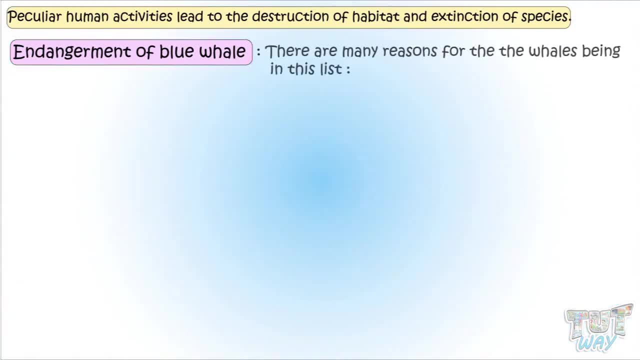 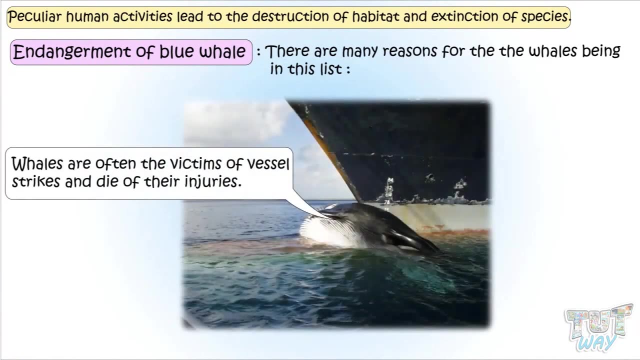 large and beautiful creature that is endangered now. ocean waters are the habitats of this beautiful creature. there are many reasons for the whales being in this list. some of the reasons are: the whales are all-terrain animals and they are the only animals that can survive in the